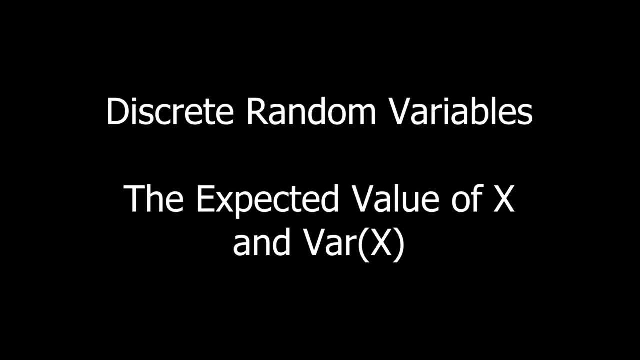 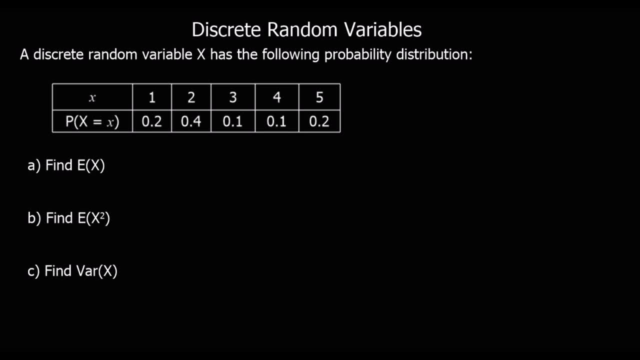 Okay, in this video we're going to look at finding the mean and the variance for discrete random variables. So the mean we call the expected value of x, So we can think of this as the mean. so the average result from this distribution and the variance we call var. 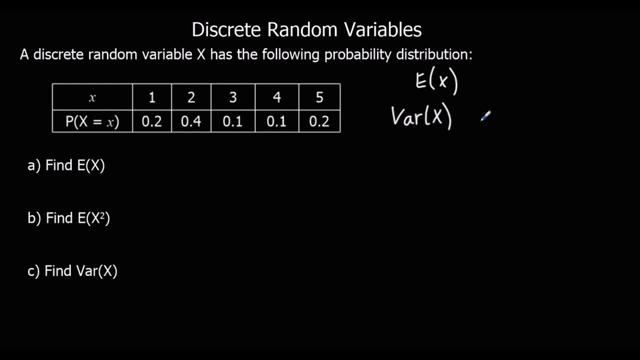 x. So that's a measure of variance for the random variable. So to find ex the expected value of x, the mean of x, all we do is we times each value of x by its probability and add them all up: 1 times 0.2, plus 2 times 0.4, plus 3 times 0.1, plus 4 times 0.1, plus. 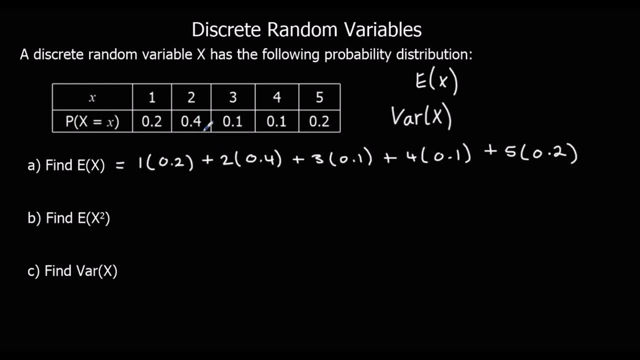 5 times 0.2.. So we can just type that into the calculator or work that out And we should get 2.2.. 2.7.. Now we're going to work out the expected value of x squared. So if all the x's were, 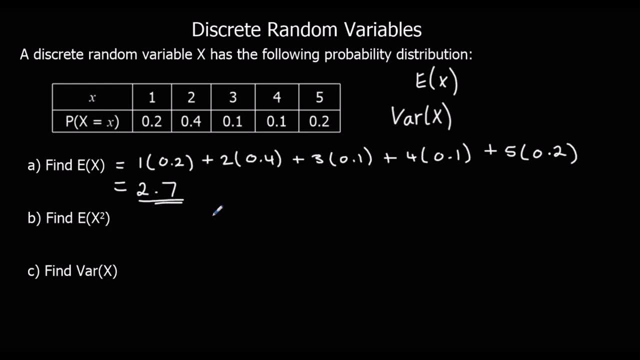 squared. what would the mean be? What would the expected value be? So it's 1 squared times the probability, 2 squared times the probability, 3 squared times the probability, 4 squared times its probability And 5 squared times its probability. So it's 1 squared times 0.2, plus 2 squared times. 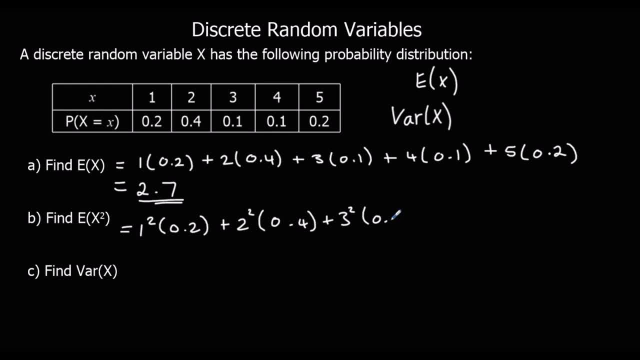 0.4, plus 3 squared times 0.1, plus 4 squared times 0.1, plus 5 squared times 0.2.. And that should give us 9.3.. 9.3.. And now var x is ex squared minus ex squared, So ex squared so 9.3 minus our ex 2.7 squared. 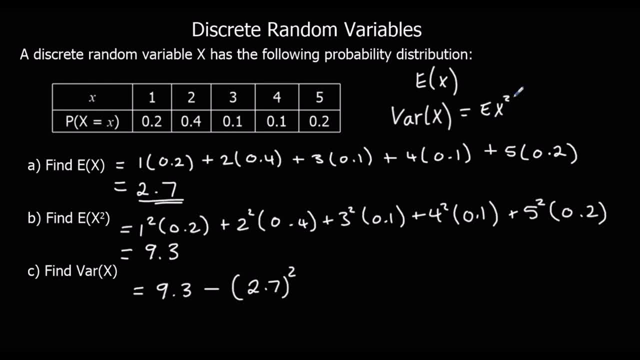 So we can say that's ex squared minus ex squared, So it's the square of the mean, The mean of the squares minus the square of the mean, like variances when we're working with other numbers. So ex squared, so this ex squared. 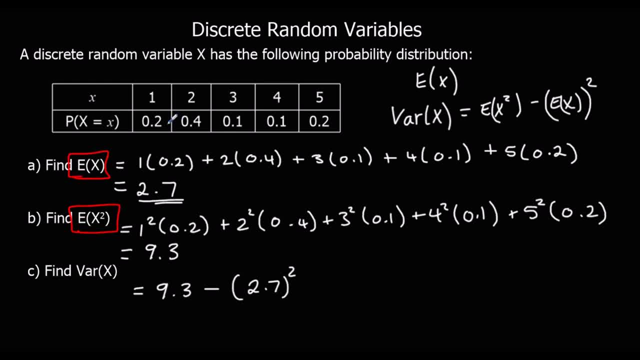 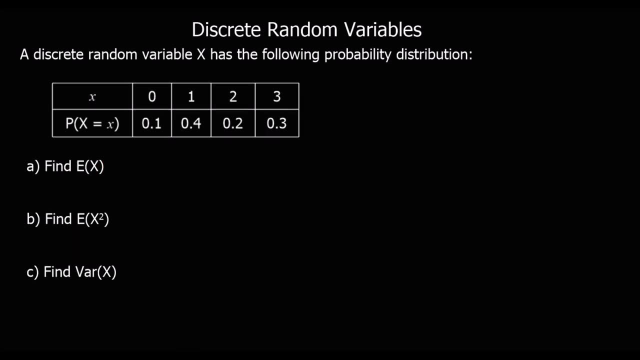 take away the mean squared, And that should give us an answer of, in this case, 2.2.. 0.01.. Okay, here's another question. So pause the video, give this one a go. So we're working out. 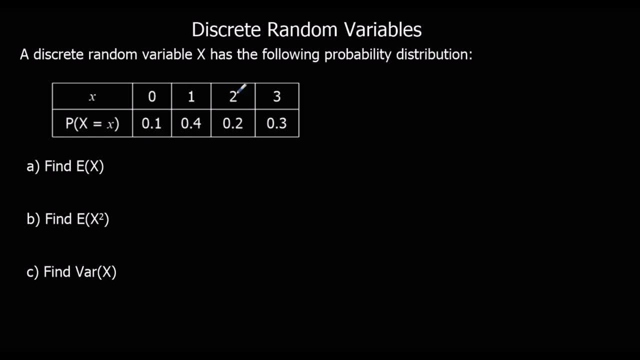 ex, which is just the mean. so times them, times them all by their probabilities and add them together. Ex squared square the number. then times it by the probability and add them all together And var x, which is the mean of the squares minus the square of the mean. 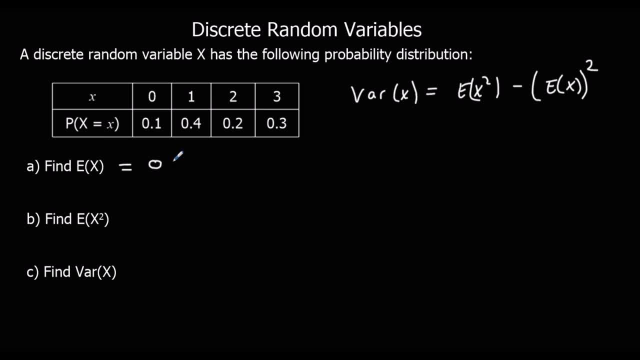 So ex expected value of x is 0 times 0.1 plus 1 times 0.4 plus 2 times 0.2 plus 3 times 0.2.. So that should give us: well, 0 plus 0.4 plus 0.4 is 0.8 plus 0.9, 1.7.. 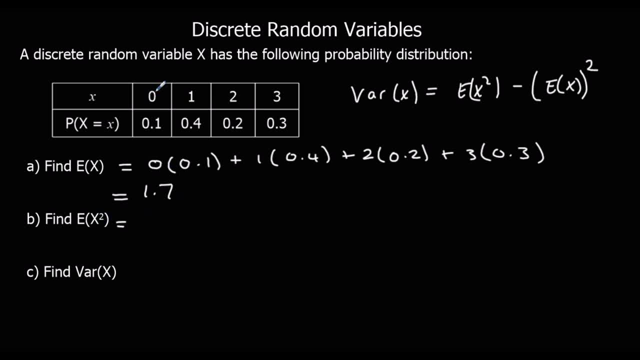 Ex squared, so it's the number squared times the probability this time. So 0 squared times 0.1.. 1 squared times 0.4.. 2 squared times 0.2.. And 3 squared times 0.3.. 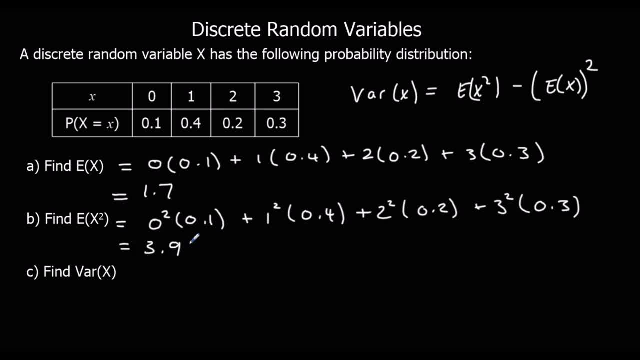 And that should give us 3.9,, which means var x is our ex squared 3.9, minus our ex squared 1.7 squared, And that is 1.01.. Thank you.